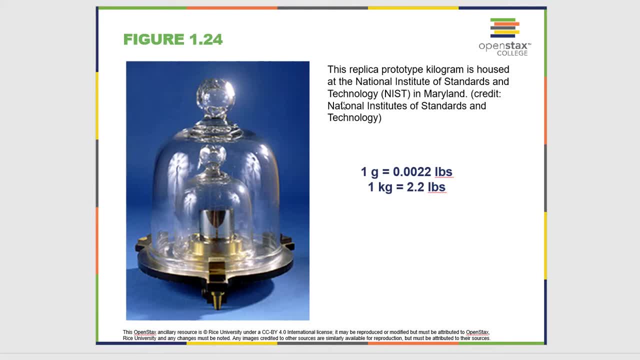 Here is the National Institute of Standards and Technology. the one kilogram mass- so this is exactly the one kilogram Mass- is essentially how much matter is in something. To give you a perspective, with the English system, one gram is 0.0022 pounds and a. 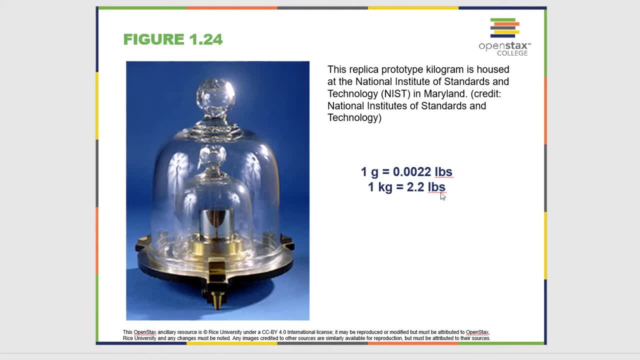 kilogram is about 2.2 pounds, So this gives you a little bit of perspective of the unit of mass. In chemistry it's very common to measure mass. It's relatively uncommon to measure distance because atoms are very small, but it's very 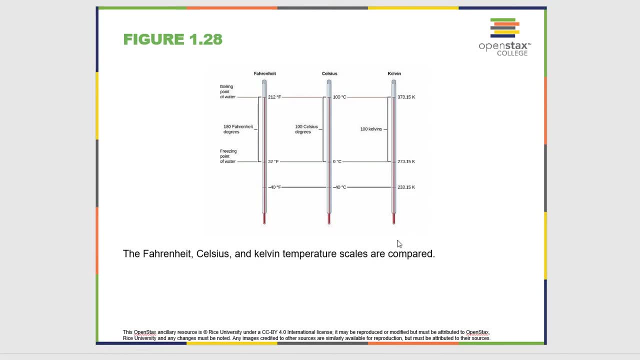 common to measure mass. Another unit we care about is temperature. Temperature has three scales that you can see compared to each other. here We have the Fahrenheit scale, the Celsius scale and the Calvin or the absolute temperature scales. Temperature is a measure of average kinetic energy, So all 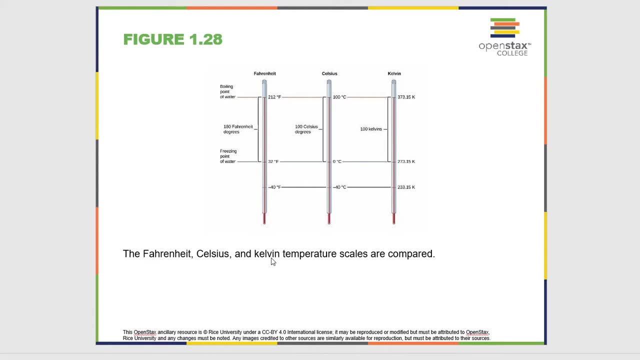 the molecules, even the molecules in something solid like the desk you might be sitting on, are moving at any temperature above absolute zero. If you were to cool these molecules down to an absolute lowest temperature, that absolute lowest temperature is the temperature at which the molecules stop. 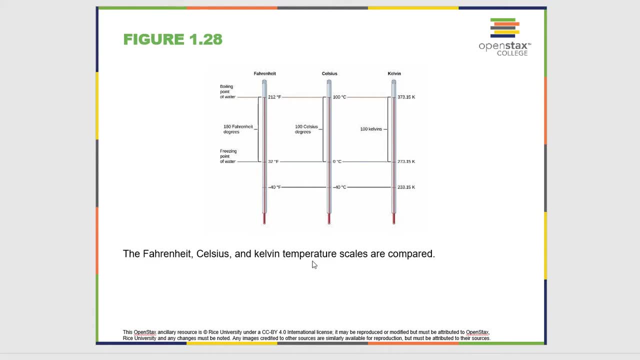 moving Now. when it comes to temperature, we do need to learn how to convert from one unit to another, and it's done slightly differently than if you wanted to convert from, say, milligrams to grams, or even if you wanted to convert from grams to pounds. these two things would be done slightly differently. So in this 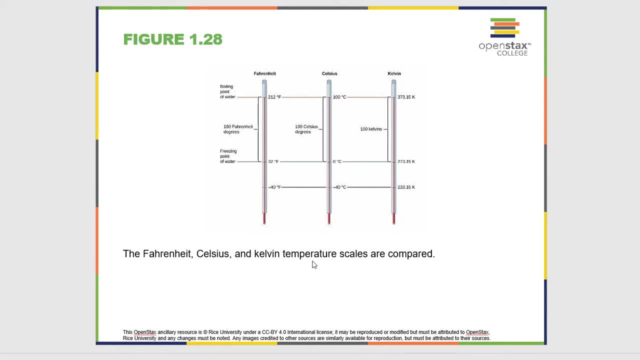 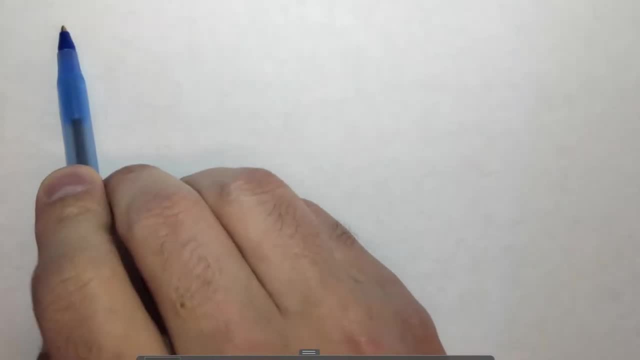 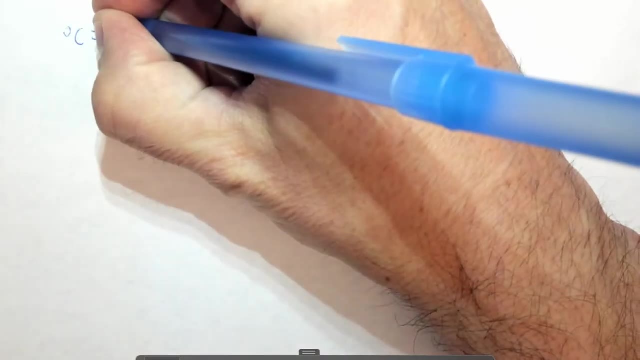 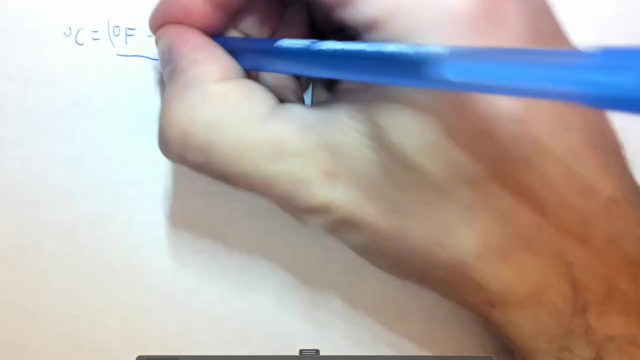 section, we do want to cover how you would convert from one temperature to another, and there are essentially three equations that you need to know in order to do this. The first is that degrees Celsius equals degrees Fahrenheit minus 32, and you do have to subtract the 32 first divided by 1.8.. You would use this. 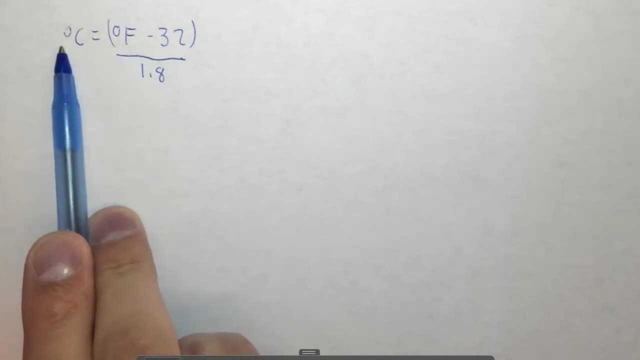 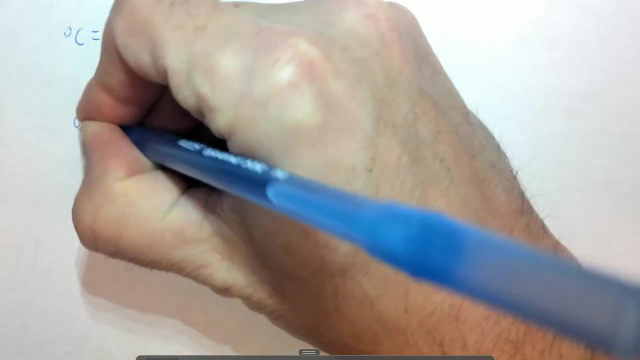 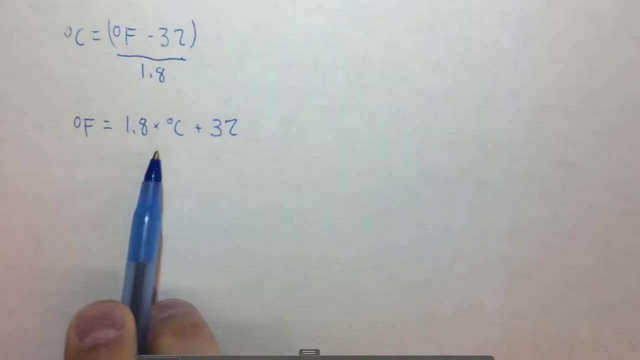 one. if you were given the temperature in Fahrenheit and you wanted to know the temperature in Celsius, The next equation that you need to know is that Fahrenheit equals 1.8 times degrees Celsius plus 32, and here it's the standard order of operations: you multiply first and then. 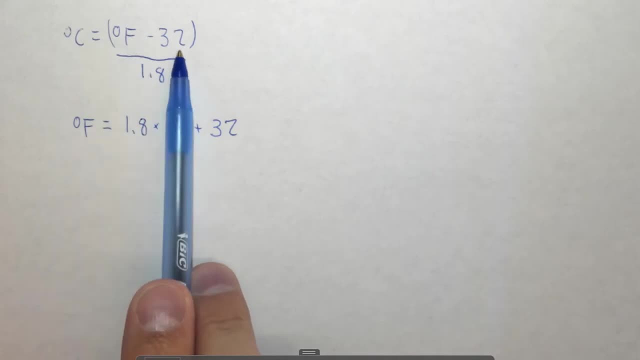 add Here the order of operations: are you subtract first and then you divide? that's why this is in parentheses, because that's the non standard order of operations, if you will. And the last one is for Kelvin, the absolute temperature scale, and Kelvin is Celsius plus 273. 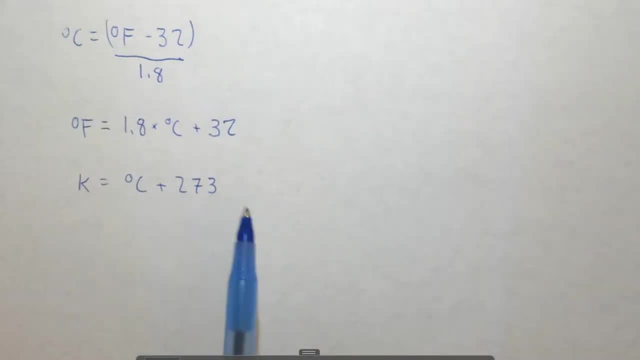 In many books you'll see plus 273.15,, although very commonly we only measure temperature to the nearest degree. So I'm going to leave off the 0.15.. If you use a typical thermometer, you usually can only get it to the nearest degree. 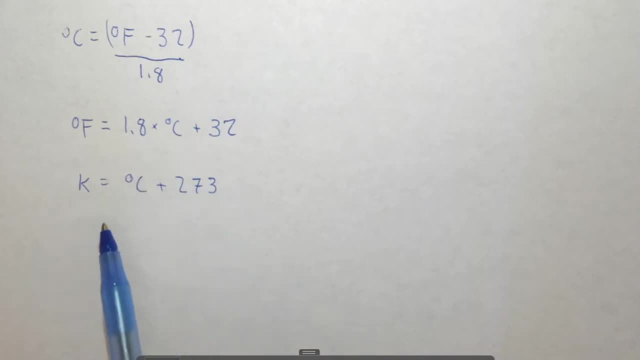 as the degree markings are very close together. Of course, there are devices that can measure it much, much, much more accurately, So sometimes you may want to use some decimal points here, But in this course, I think this is good. So let's pick some common temperatures and let's convert them to different units. 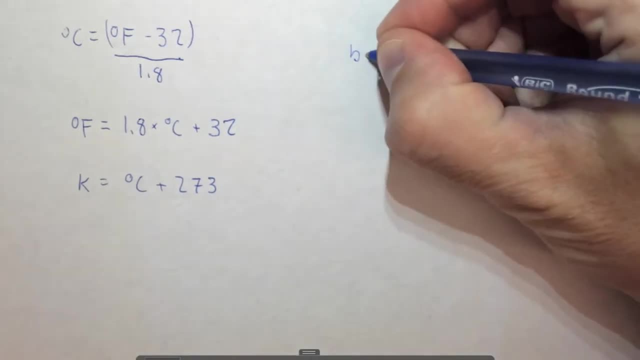 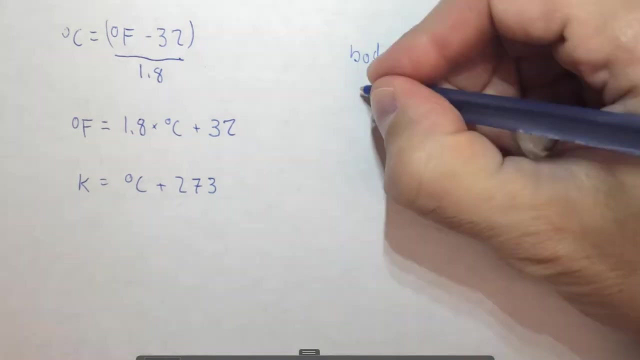 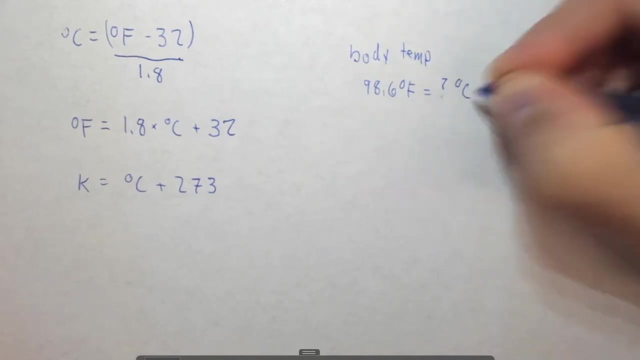 So let's take body temperature. Body temperature is a common temperature that we're all familiar with, And in the United States we're familiar with this in Fahrenheit, which is 98.6 degrees Fahrenheit. Let's say we want to know what that temperature is in Celsius. 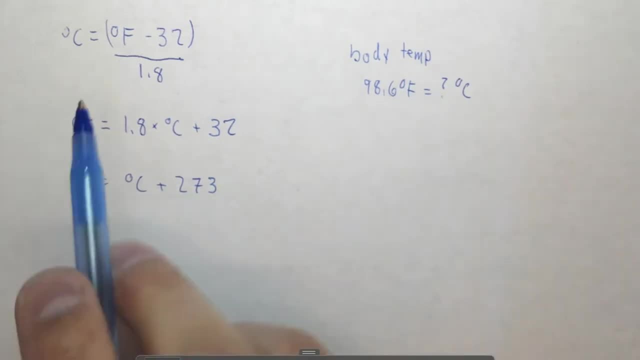 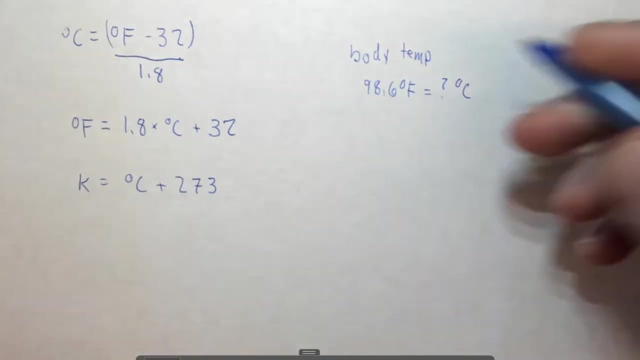 So this could be a question on the homework. So if we want to know what it is in degrees Celsius, we'd use the equation where decreased Celsius is by itself. So degrees Celsius equals the Fahrenheit degrees 98.6, minus 32, divided by 1.8. 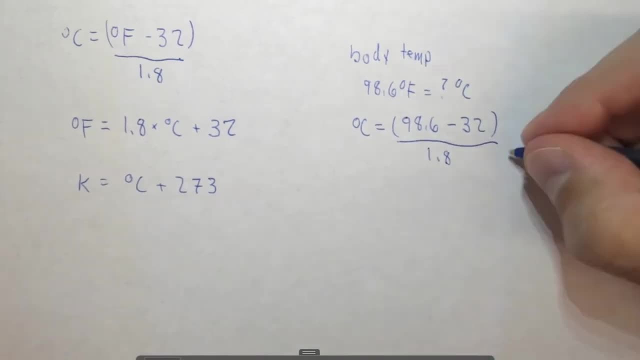 And, as I mentioned before, you need to subtract first and then divide, And when you do this you get 37 degrees Celsius. You could argue it's 37.0 degrees Celsius. We'll talk about significant figures later on, So this is important for right now. 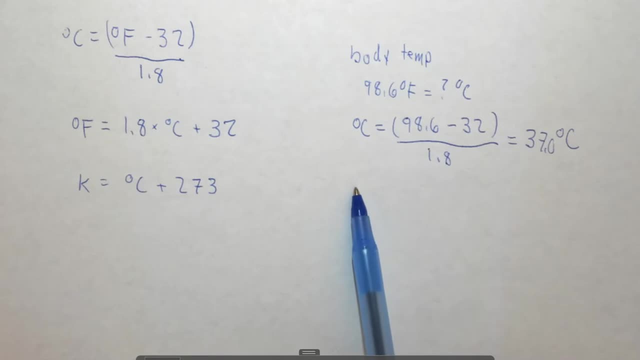 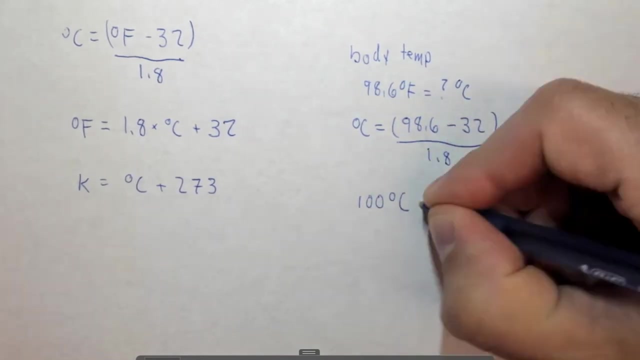 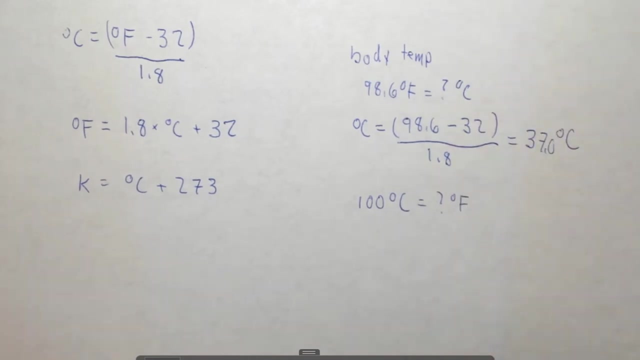 That's coming up in this chapter. however, Let's look at another example. Let's look at the boiling point of water. Water boils at 100 degrees Celsius. What is that in Fahrenheit, for example? So, in Fahrenheit, 100 degrees Celsius. 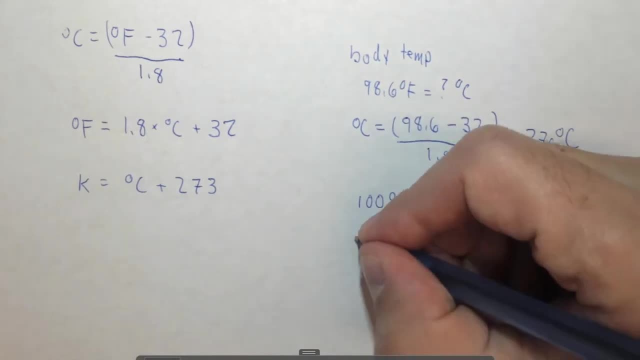 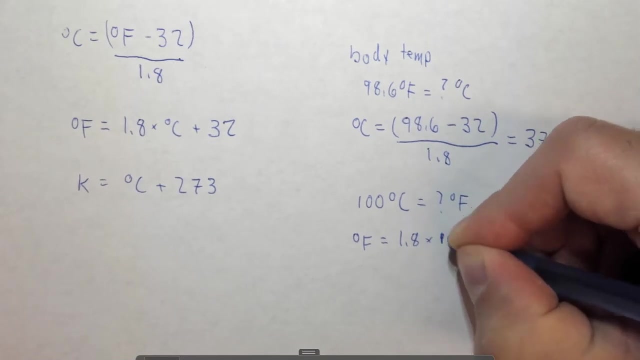 We would have to use this equation because Fahrenheit's by itself. So we take: Fahrenheit equals 1.8 times 100 plus 32.. And, as you may know, the boiling point of water in Fahrenheit is 212 degrees Fahrenheit. So we converted from Celsius to Fahrenheit. 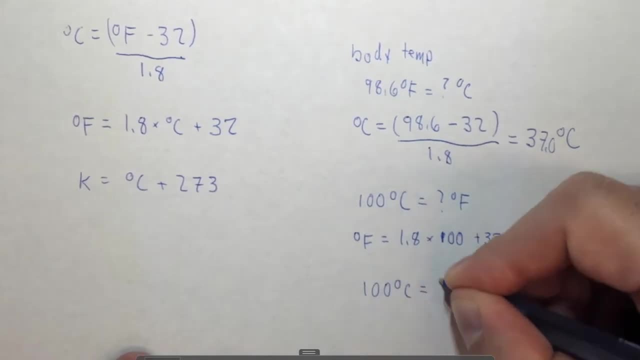 What if we wanted that same temperature, 100 degrees Celsius in Kelvin? Well, we could figure that out. We could figure that out as well: Kelvin equals the 100 degrees C plus 273, which, of course, is 373 Kelvin. 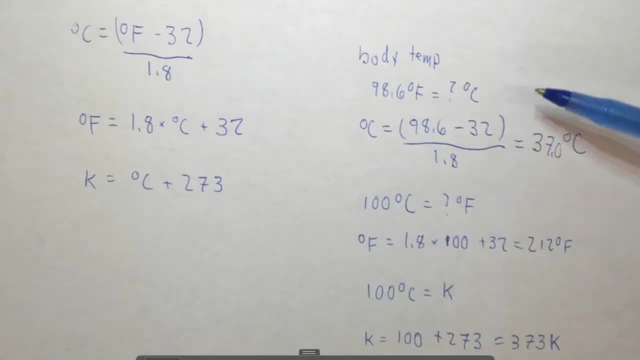 So we do need to be familiar with how to convert from one unit of temperature to another unit of temperature, And this is how these equations are, how we could do this. These are a good thing to write down so that you have them handy when you need them. 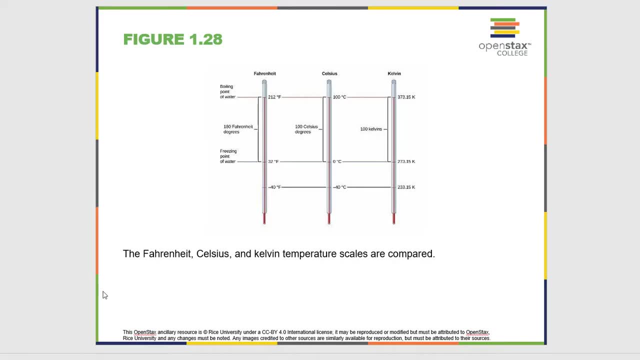 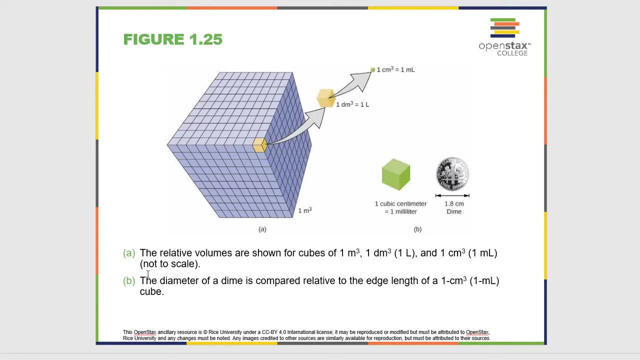 Another. Another unit of measure is volume. Volume is a unit of measure that we commonly use in chemistry, And volume is a three-dimensional space. So if you take a one centimeter by one centimeter, by one centimeter cubed, you would actually have a milliliter. 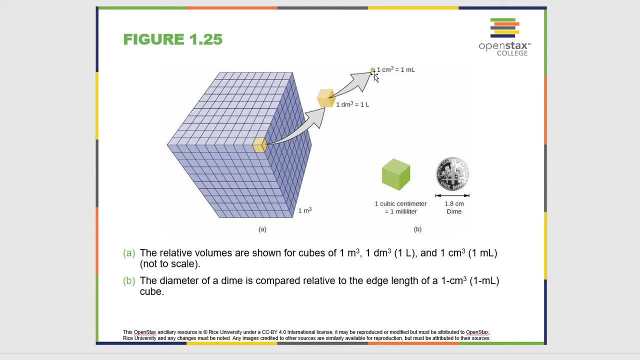 And this is not one centimeter cubed. This, I guess, is supposed to represent the one centimeter. But one centimeter cubed is defined as a milliliter, One decimeter cubed is defined as a liter, And then a meter cubed doesn't have a meter. 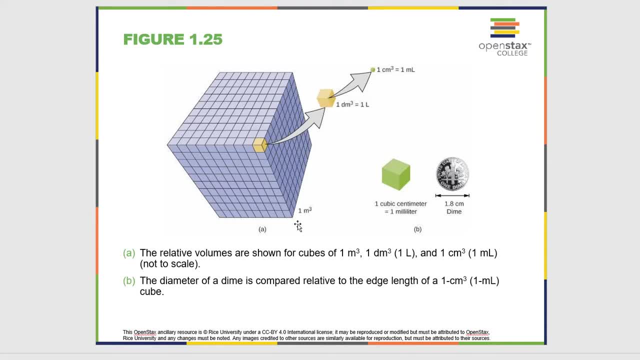 It'd be multiple liters, Okay In volume. So these are some examples. Note that a centimeter cubed equaling a milliliter is something you definitely need to be familiar with. You should also note that a centimeter cube is sometimes called the CC. 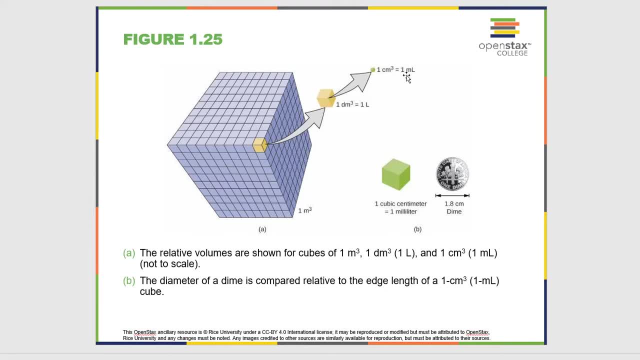 So, for example, if you were in a hospital setting, they might say: you know. if you were in a hospital setting, they might say you know the patient needs five CCs of whatever. Well, five CCs and five milliliters are the same thing. 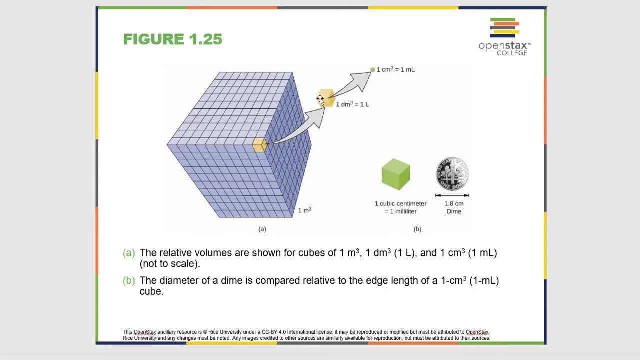 So if you have a three-dimensional space, that's one centimeter by one centimeter by one centimeter, that is defined as a milliliter. You could also have kiloliters, You could have liters, You could have the same thing you could have with the prefixes. 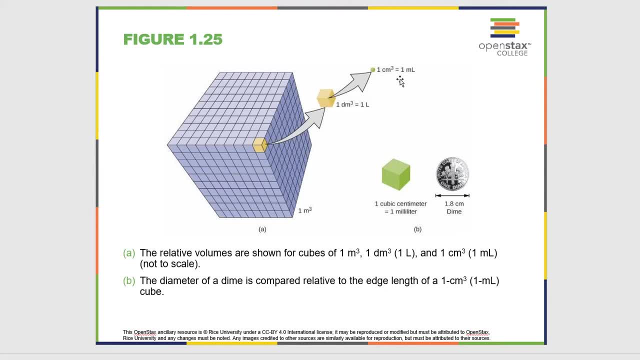 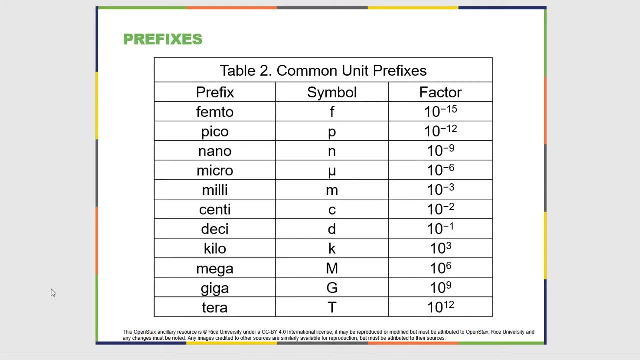 in the other cases- And we'll talk a little bit more about the prefixes in a couple of minutes- When you have units of measurement. when you have units of measurement, one thing that you have to be concerned about is sometimes you have very, very small. 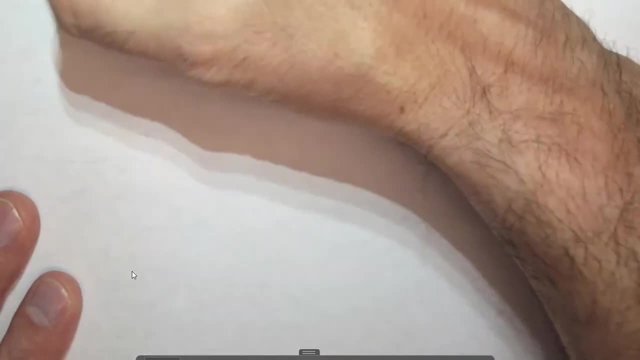 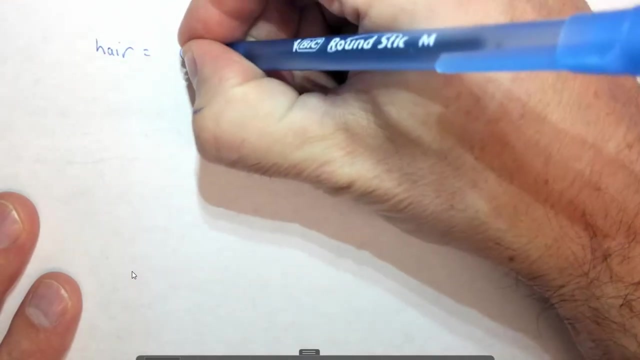 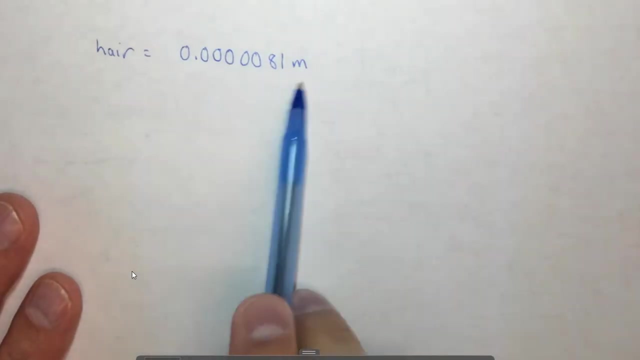 and very, very large measurements. So let's say that you have a hair, A human hair, And the diameter is 0.0000081 meters. So this is the diameter of a hair. Or let's say that you have the distance. 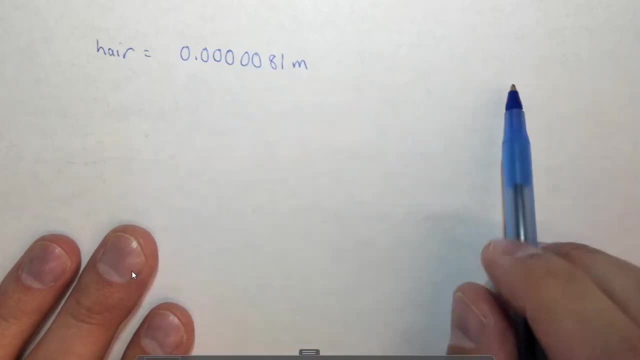 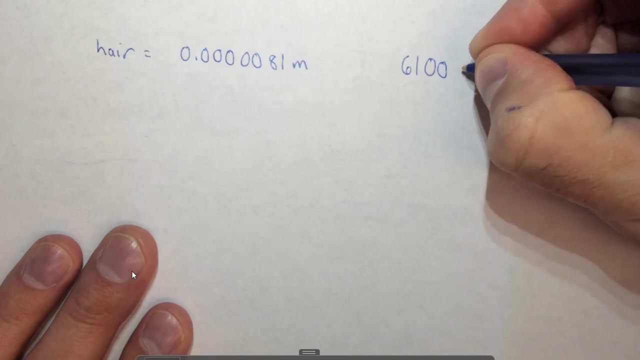 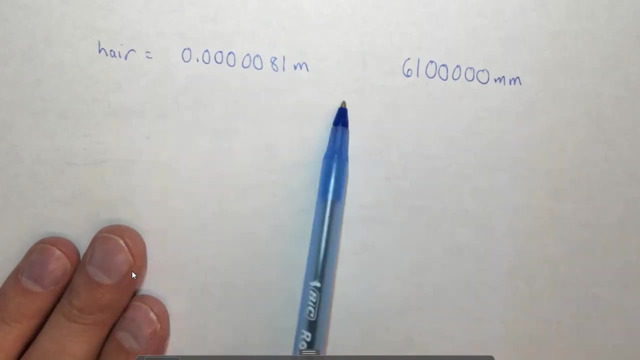 between the uptown campus and the downtown campus at the University of Albany in millimeters, Which is 61, 1, 2, 1, 2, 3 millimeters. So I was just counting the zeros there. So these units are. 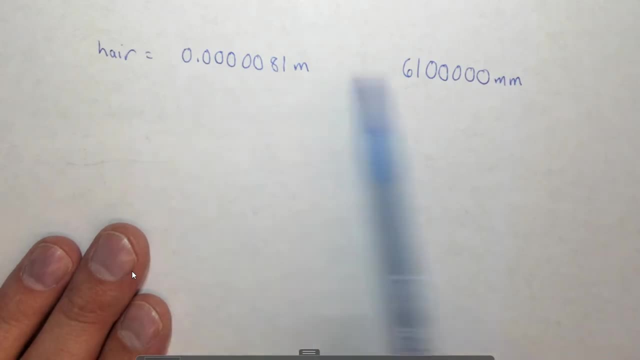 very, very. in this case, a very, very small unit And in this case, a very, very large unit. It's a lot of millimeters Between the uptown campus and the downtown campus at UAlbany. In fact, it's 6.1 million. 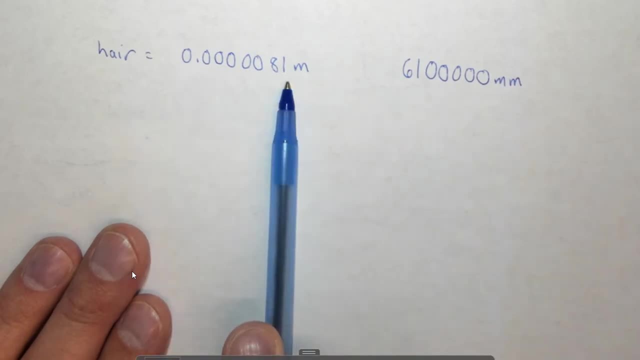 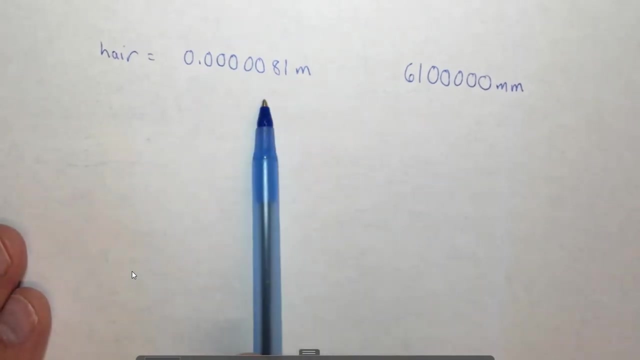 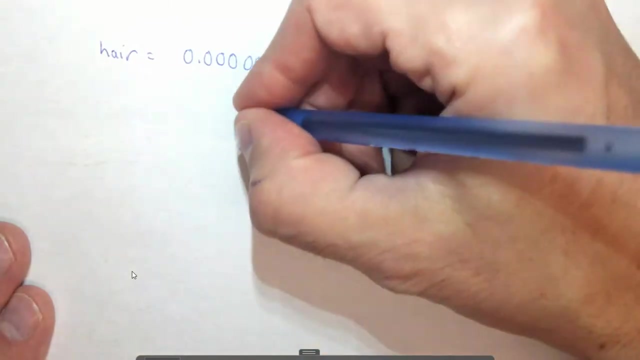 millimeters. It's a very small number of meters between the university or, excuse me, for the diameter of a hair. So here we use something to express these numbers. There's actually two ways we can do this. One way we can do this is to express: 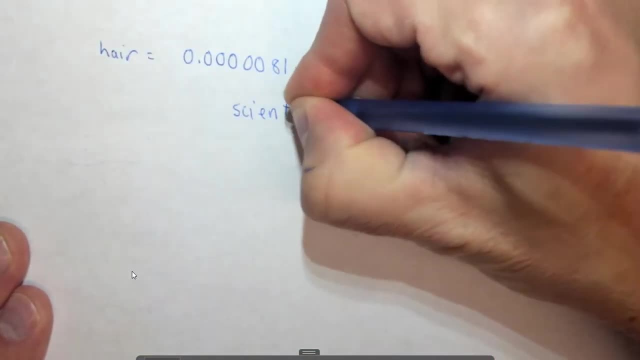 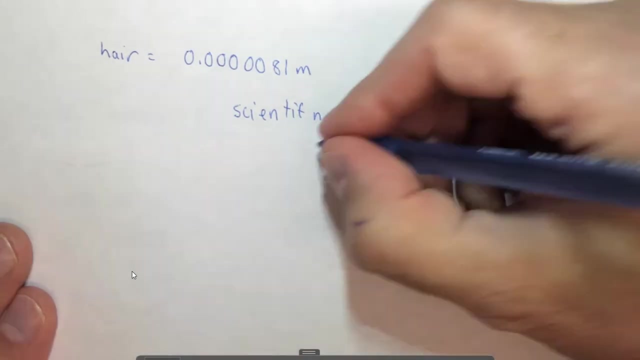 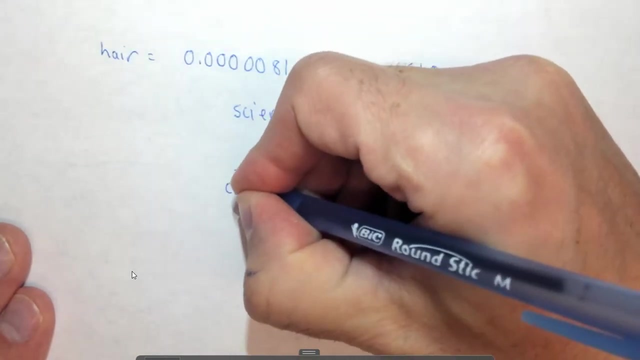 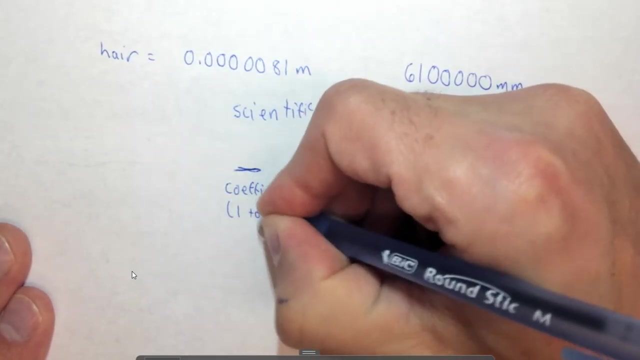 these numbers in scientific notation. So scientific notation consists of two parts. First, I should finish writing the word. Scientific notation consists of two parts: The number out here, which is called the co-efficient, Which has to be between 1 to 9.9. 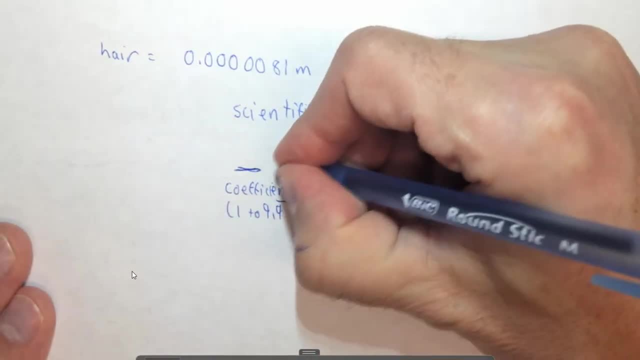 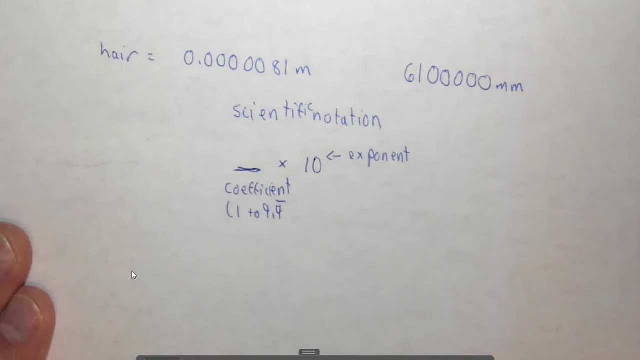 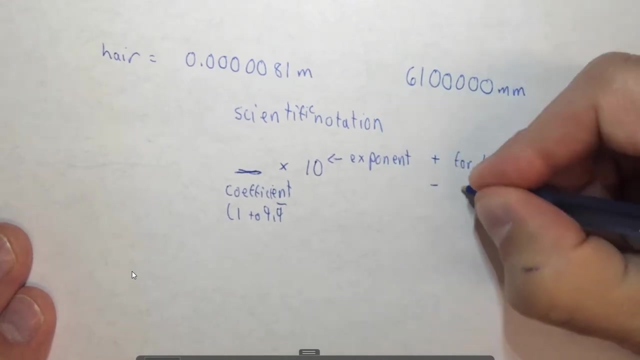 repeating by definition. Then we have times 10 and up. here we have an exponent, so a superposition of a prescripted number which is positive for large numbers- and here we define large numbers as greater than one- And negative for small numbers, which here we define. 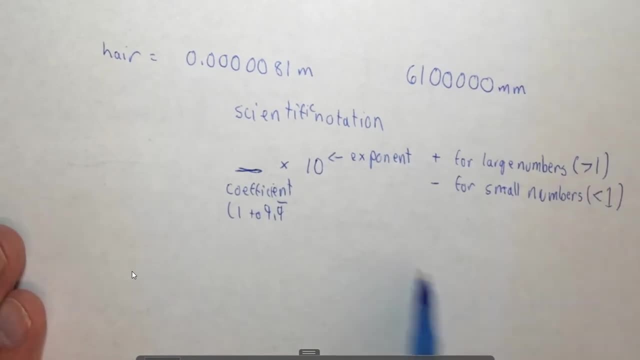 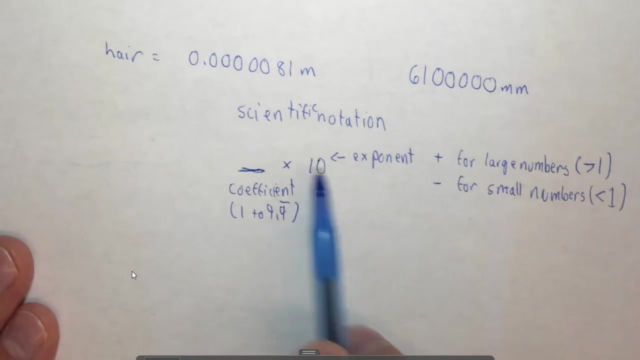 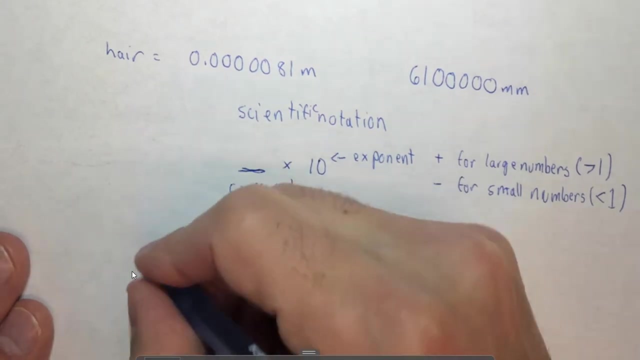 as less than one. So these are the components. So we have an exponent which must be between 1 to 9.9, repeating times 10 to some, exponent which is positive for large numbers and negative for small numbers. So let's look at our first example. 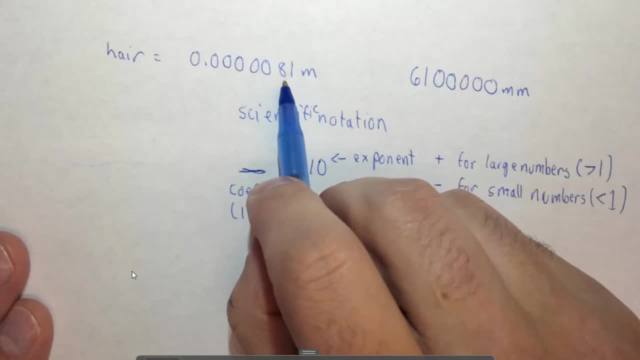 Let's look at this number here. So we want to express this in scientific notation. So we need to make this .000081 meters into something that is between 1 and 9.9.. That number means we need to put the decimal place between: 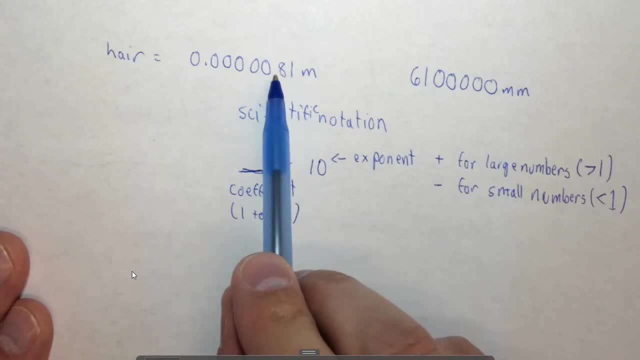 the 8 and the 1., So we get 8.1.. We can't use .81, because that's less than 1.. We can't use 81, because that's greater than 10.. So we have to use 8.1.. 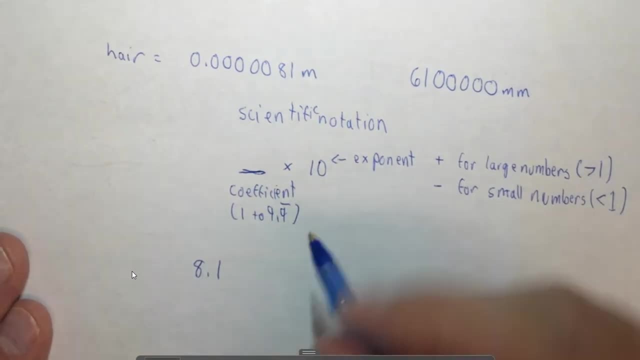 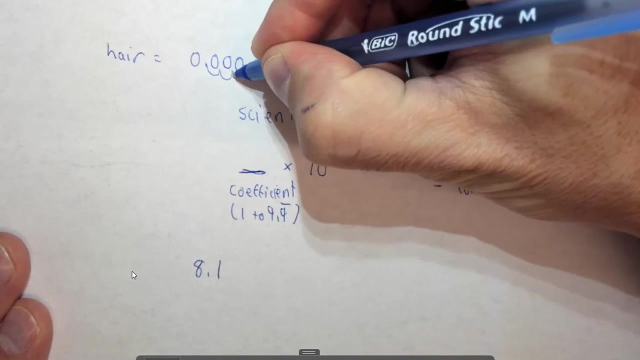 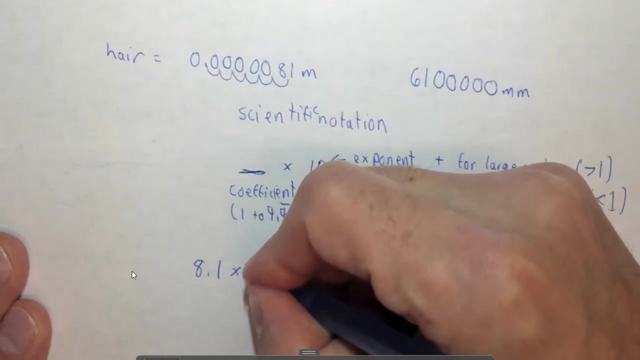 So we use 8.1. Now the decimal place starts here. How many times do we need to move it? We need to move it 1,, 2,, 3,, 4,, 5,, 6 times. So we need to move it 6 times. 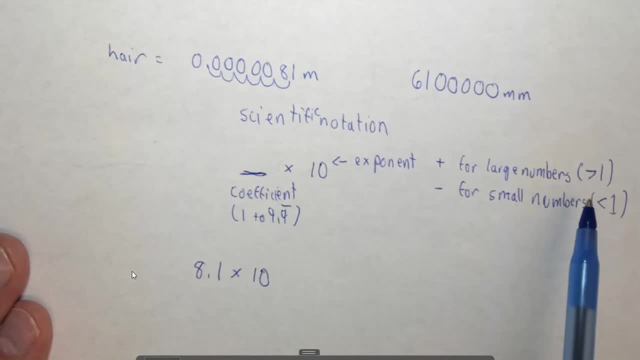 Times 10.. Is it negative 6 or positive 6?? Well, in this case it is going to be a small number. This is less than 1.. So it's negative 6 and the meters stays. So we have 8.1 times 10 to the minus 6. 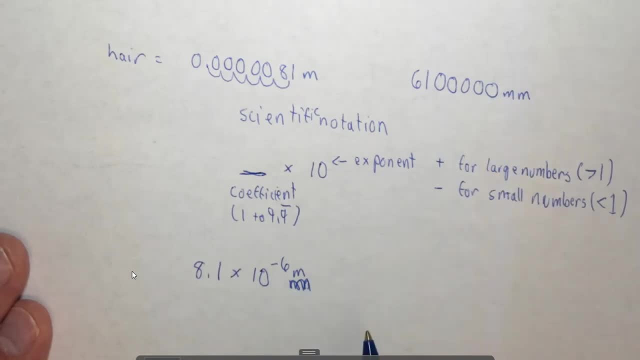 meters. Let's look at this example here. In this case, the number that we need to write is 6.1.. It can't be 61.. It can't be 61 because it has to be 1 to 9.9.. So it's going to be. 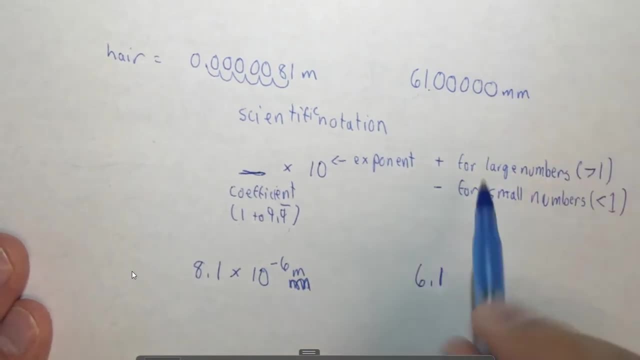 6.1 as the number. Well, here we don't have a decimal place. So if a number doesn't have a decimal place, we assume it's at the end. Now, how many times do we have to move it in order to make 6.1?? 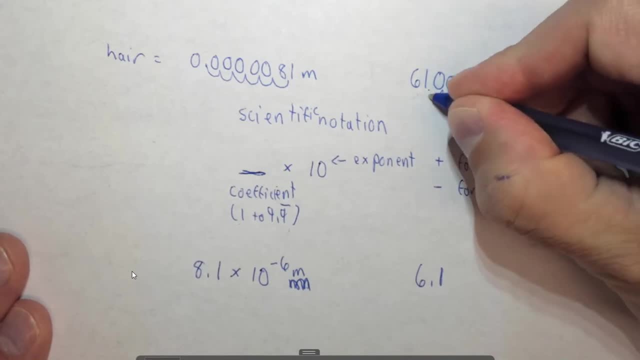 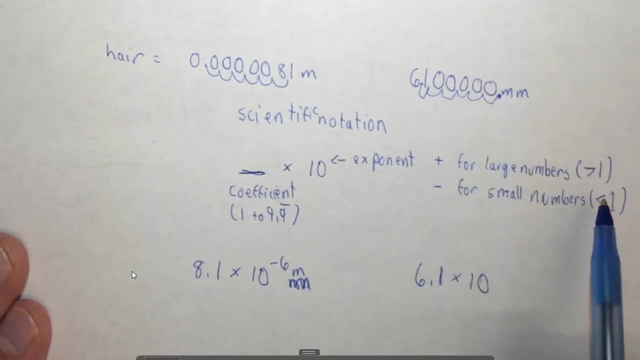 Well, we have to move it 1,, 2,, 3,, 4,, 5, 6 times. By coincidence, they're both 6. Times 10 and then, in this case, it's a large number. We started with 6.1 million. 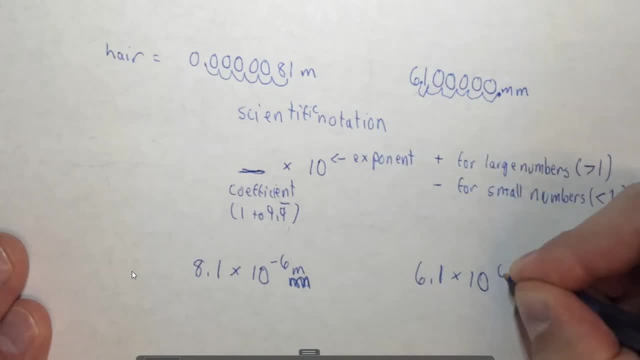 and that's certainly greater than 1.. So it's 6.1 times 10 to the 6 millimeters. So these numbers are expressed in scientific notation. It's a very good idea to practice this a few times so that you know how to express very small. 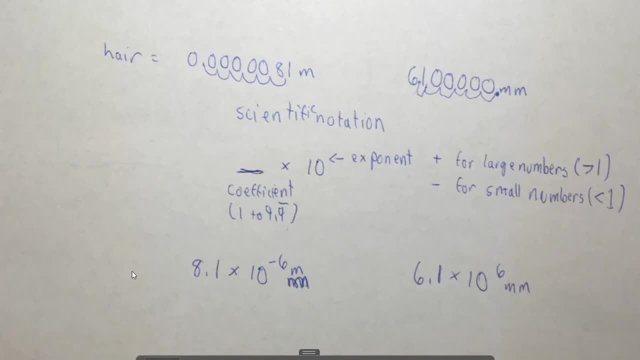 and very large numbers in scientific notation, And in fact scientific notation is useful for exactly that. This is kind of a pain to write and understand. This is much more straightforward to understand and that's why we use scientific notations. But there are 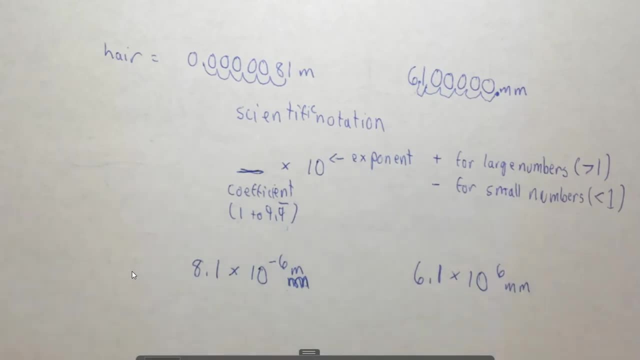 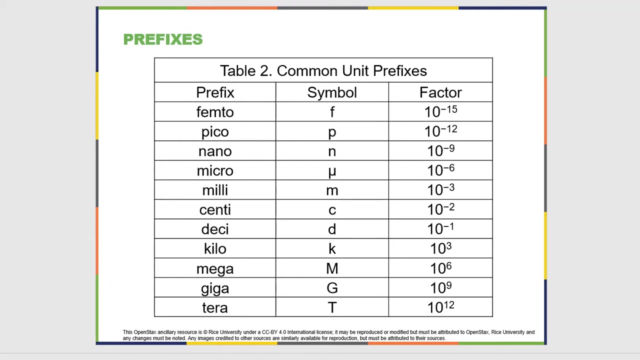 rules, and those rules are outlined here. So this is scientific notation. Another way to do this is to use different prefixes. So these are some prefixes which you may want to refer back to in order to do the homework, for example. So some of 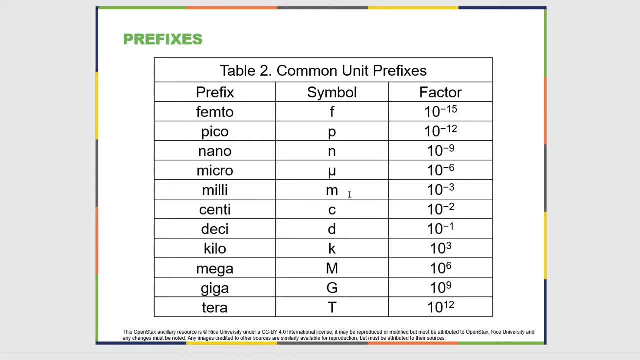 these you've heard of like millimillimeters, OK. centi. centimeters, OK kilo. kilometers or kilometers Pronounce the same thing. Some of them are used in the computer industry. Mega, which means a million, So a megabyte. 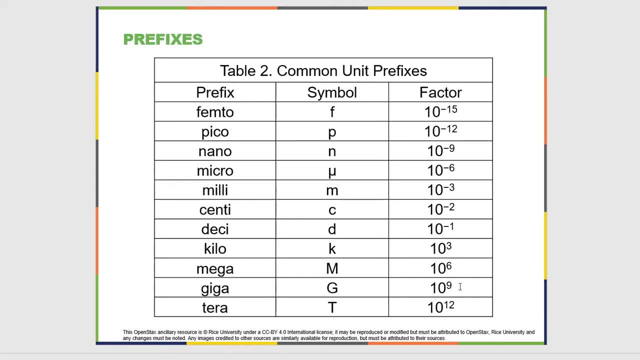 is a million bytes, A giga, which means a billion, So a gigabyte is a billion bytes And tera. now these things are becoming more common. A terabyte hard drive, which is 10 to the 12 bytes, It's a thousand times more than a. 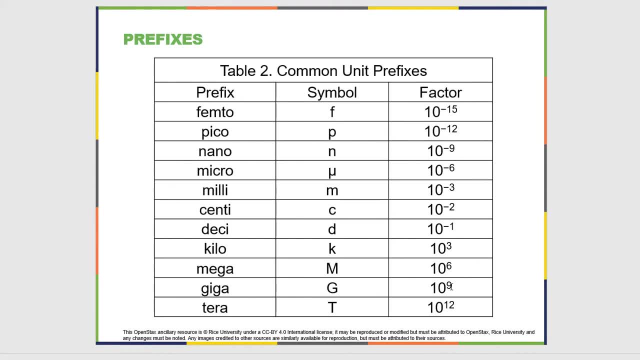 billion. So that's a tera. So that's some examples from the computer industry. You may have heard of nanotechnology. Nanotechnology is 1 times 10 to the minus 9 meters. This is in the realm of the distance between: 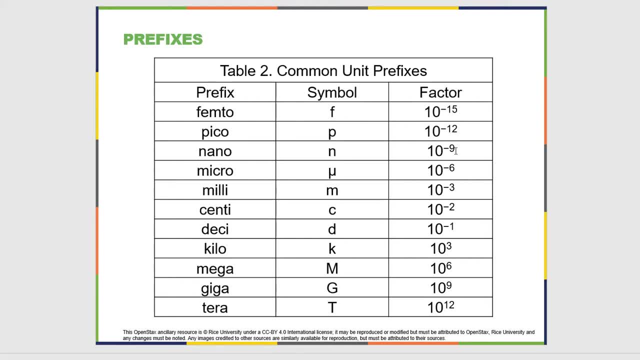 atoms. It's not quite bond distance or something like this, but it's in the realm of those sizes. So I don't know. 50 or 100 atoms might be in the size of a nanometer, put edge to edge. 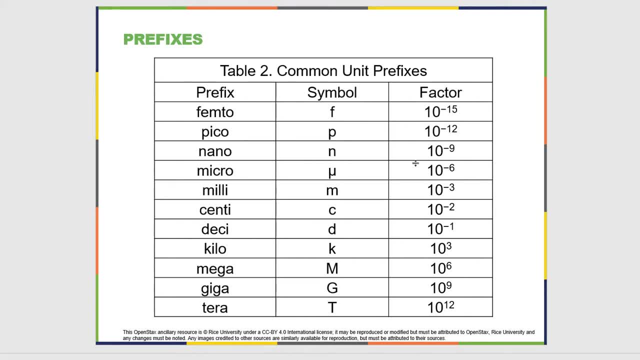 depending, of course, on how big the atoms are. So these are some different units that are used, And in the next section we'll talk a lot about how to convert from one of these units to another. But here I just want to give you an example. 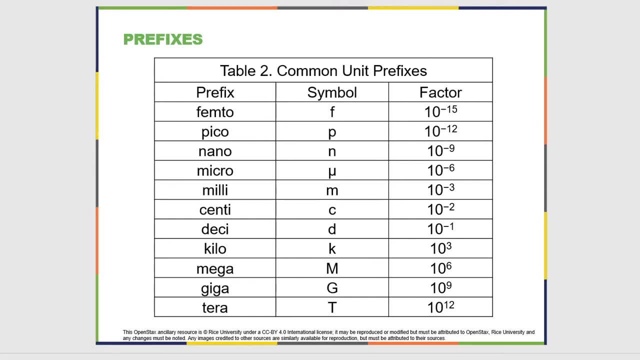 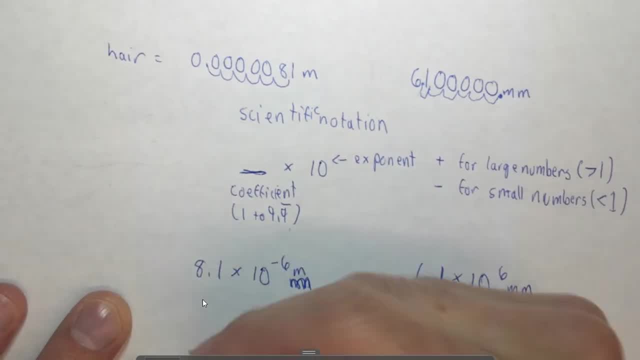 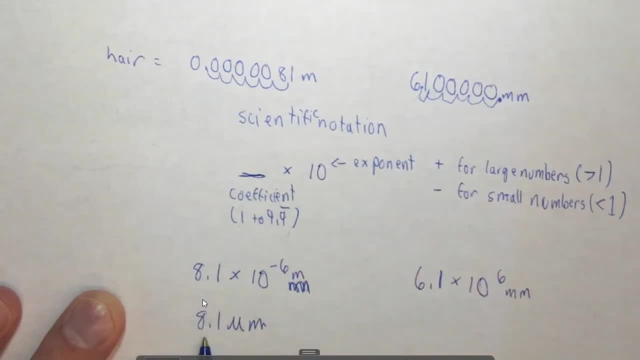 of how this might relate to the previous case. So another way of expressing this, 8.1 times 10 to the minus 6 meters, is to call this 8.1 micrometers. And this and this are the same distance. So if, for example, 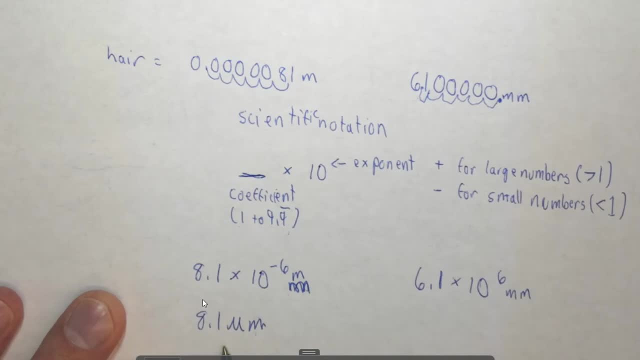 we were measuring the width of a hair. we might want to do it in micrometers because it's more convenient. We get 8.1 micrometers and then we don't have to write this in scientific notation And this, if you recall, is the distance. 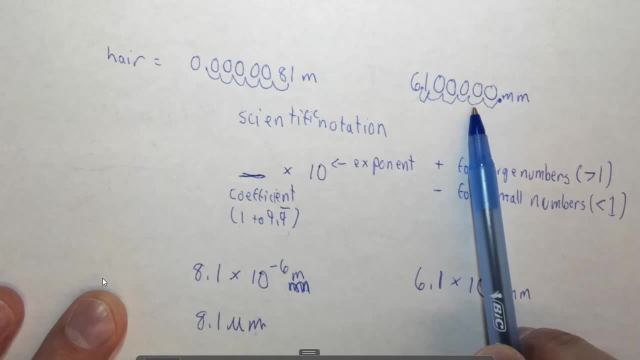 between UAlbany Uptown Campus and Downtown Campus, And this is certainly not going to be expressed in millimeters. If you lived in another country besides the United States and you looked this up on Google Maps, for example, the distance between 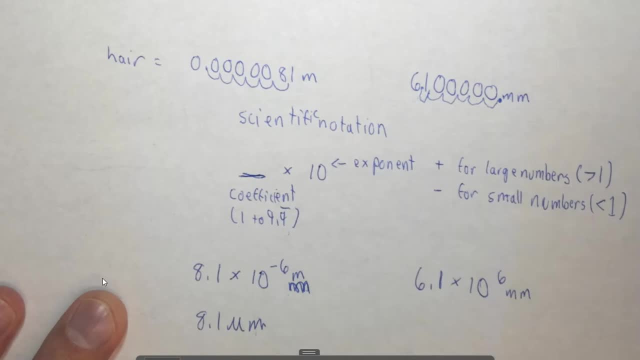 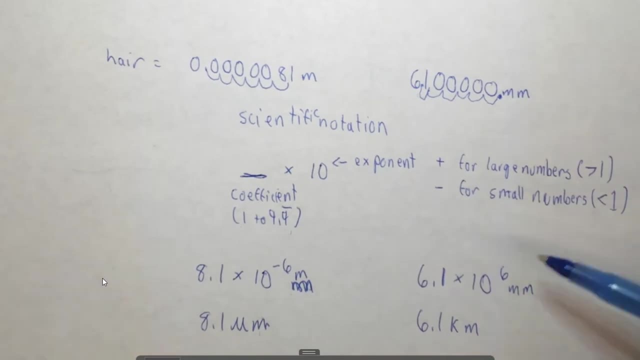 one part of a city and another part of a city is measured in kilometers, That's a common unit of distance. So this is 6.1 kilometers. So the reason that all of these prefixes exist is because they're convenient for different things. If you're measuring the distance, 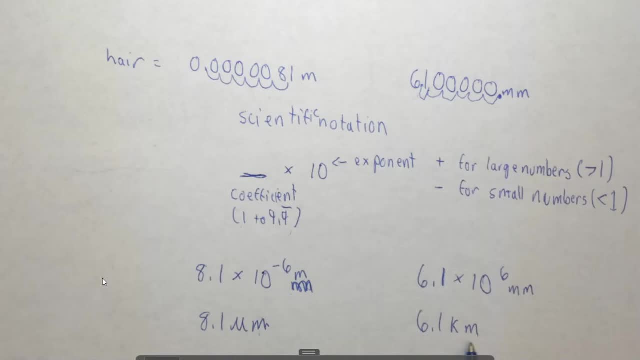 between two points in a city, kilometers is a good unit. If you're measuring the width of a human hair, kilometers is not a good unit. Micrometers is a good unit, Maybe even millimeters, which was the original unit, which was bad for the distance between two cities. 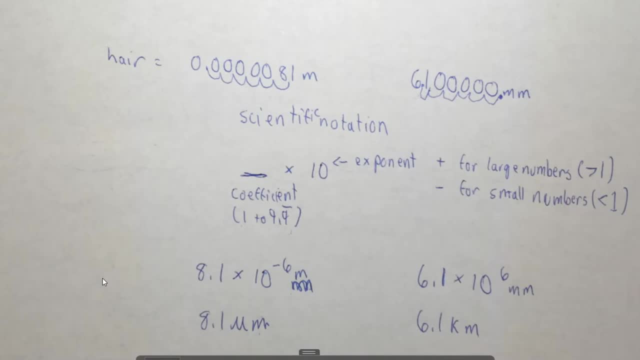 but even millimeters would probably be better than meters, But micrometers is probably the most appropriate. So that's why all of these different things exist. In the next section, as I mentioned, we'll talk in more detail about how to convert from, say, 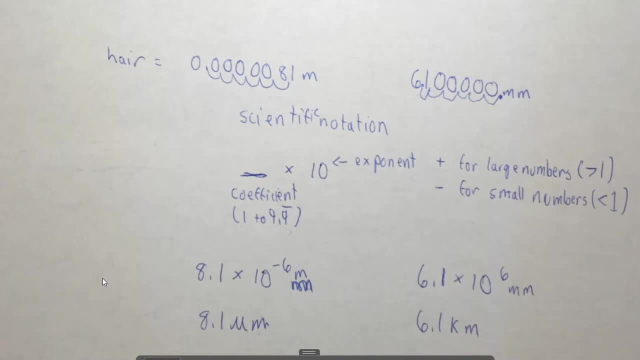 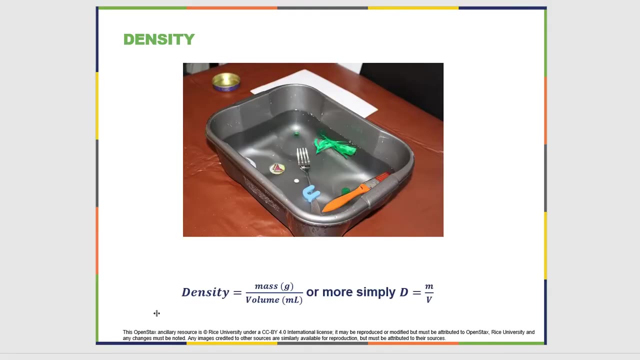 this number, to this number, because that's an important point in chemistry. So the next thing that I want to talk a little bit about is density. So density is equal to the mass divided by the volume, Or, more simply, d equals m over v. 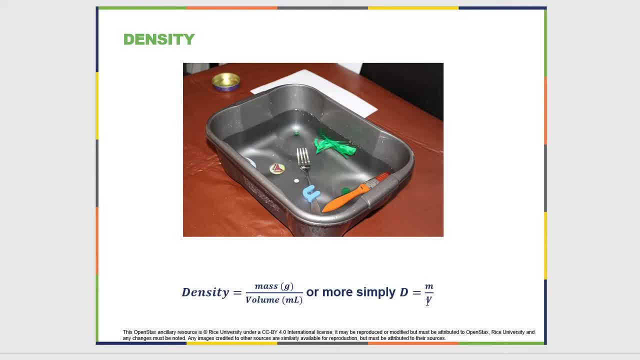 This is a ratio between the mass of an object and the volume of an object And is a common property that we use in chemistry and we measure In fact in the lab. if you take the lab here at UAlbany, you will actually measure. 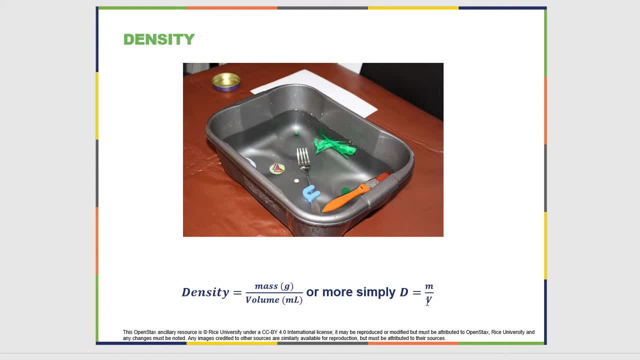 the density of sugar water solutions and use it to find the amount of sugar in Coke or some other commercial soft drink. So here we have density equals mass divided by volume. So if we look here we have a pail of water and you can see some objects. 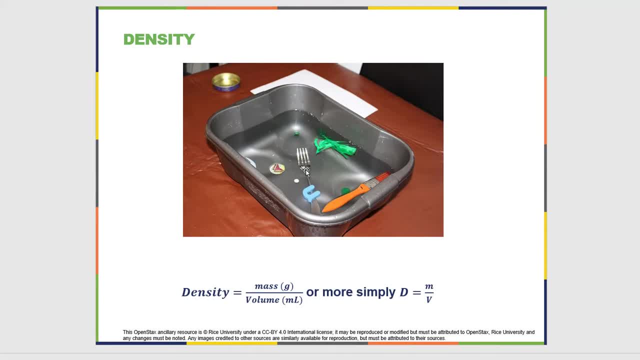 are more dense than water. So a fork which may be made out of iron, for example, Iron is more dense than water, so the fork sinks. This letter U is probably made out of some kind of foam, which is some kind of plastic. 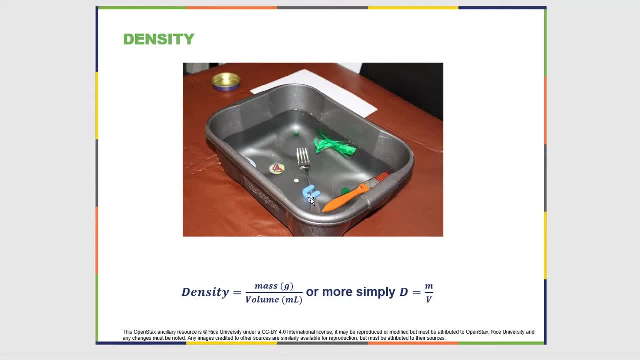 polymer or carbon polymer, And it tends to be less dense than water, So this U floats. This paintbrush is made out of several things, one of them being wood. Wood is less dense than water, so this floats. So objects layer themselves based on density. 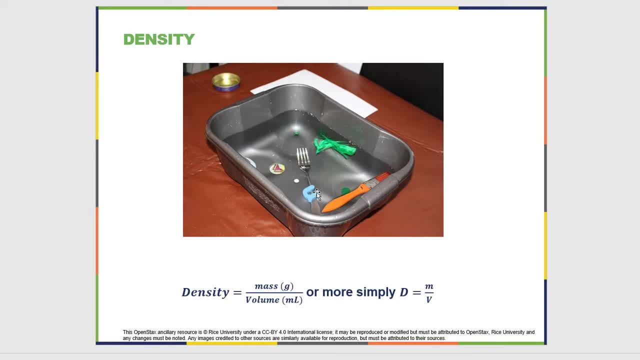 So if you look at the earth, the water tends to be on top of the soil, like in the ocean. Underneath the ocean there's a bottom which is soil. Soil is more dense than water, so water is on top. 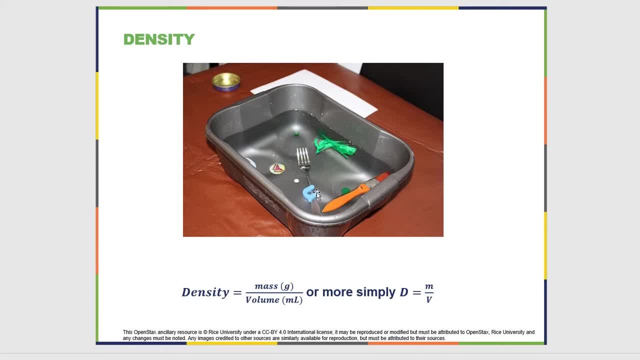 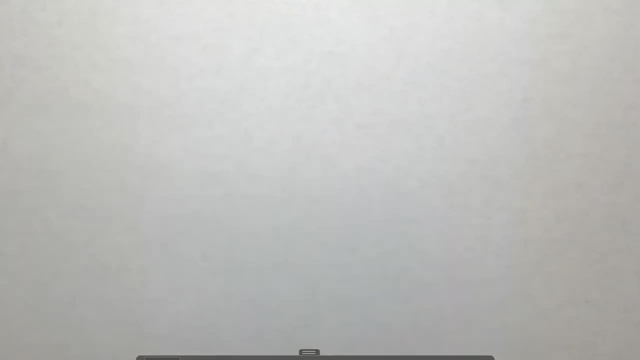 Water is even less dense, So the air is above the water and is above the soil. So these are just some examples of how things order themselves based on density, and how they sink. As one quick example of density, I wanted to look at gold. 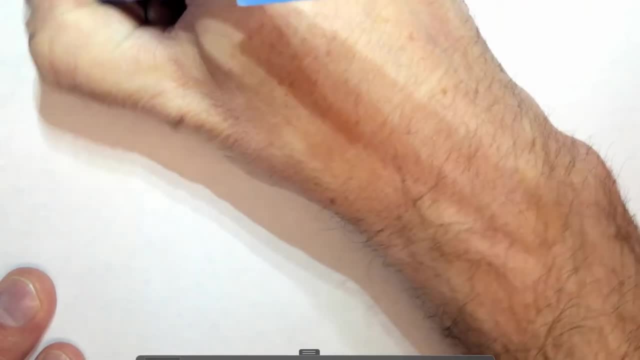 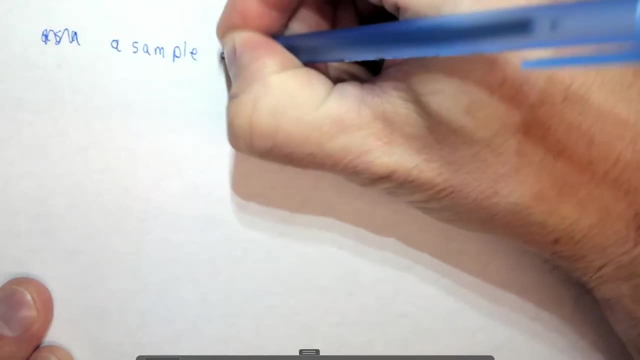 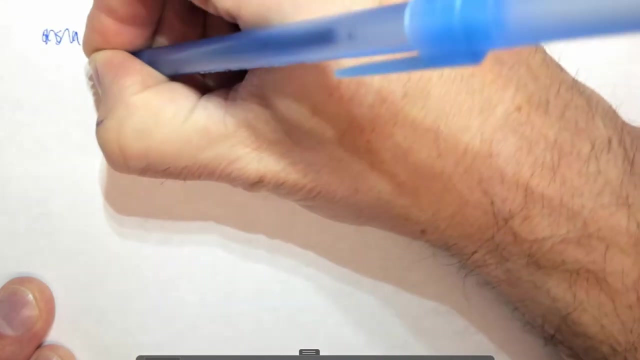 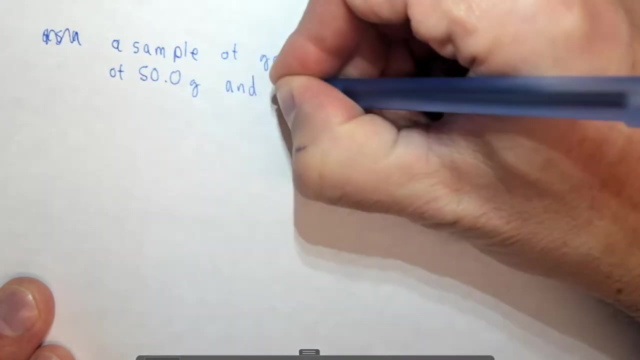 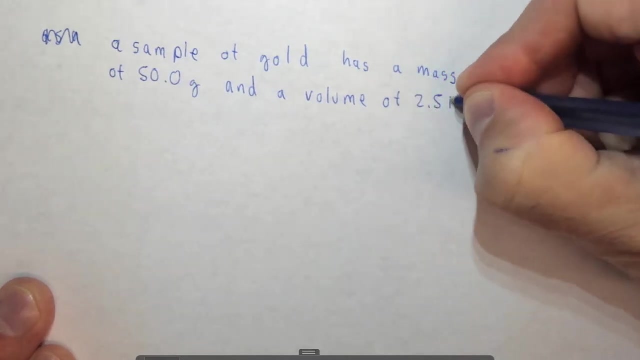 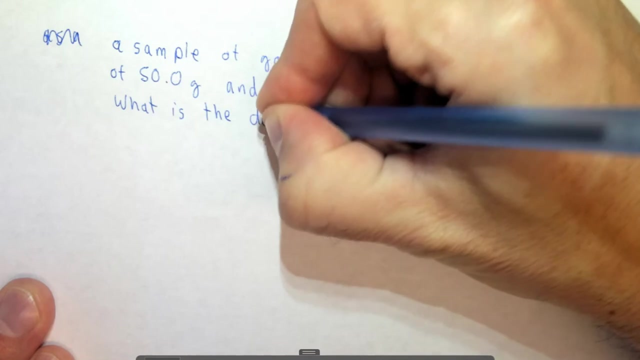 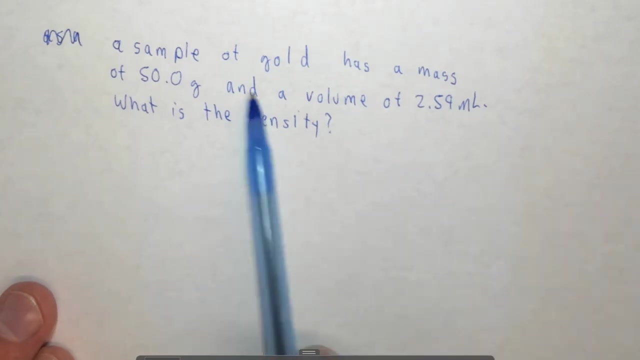 A sample. I need to put this on the screen. a sample of gold has a mass of 50 grams and a volume of 2.59 milliliters. What is the density? Alright, so we want to find the density of the gold, And it turns out that gold 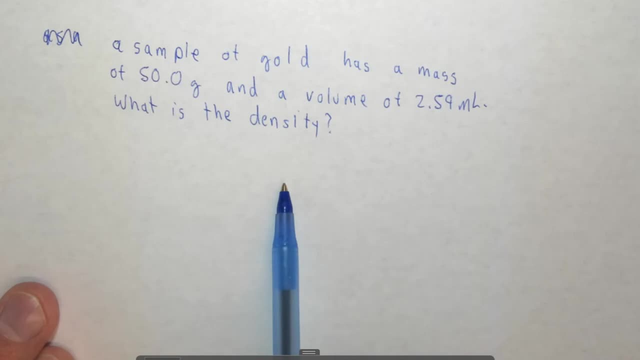 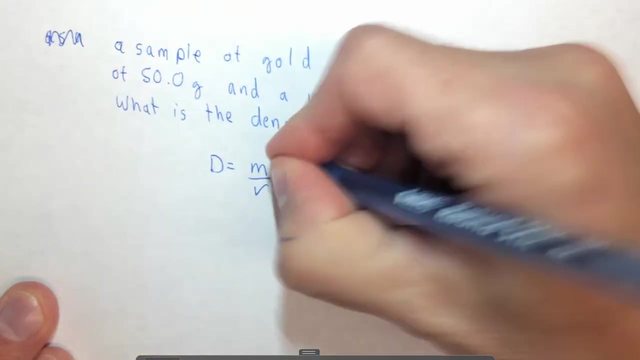 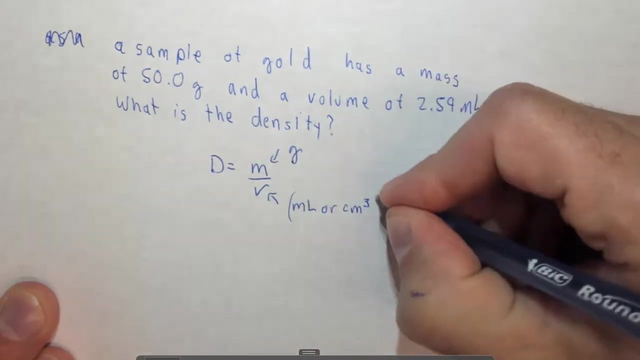 is one of the most dense substances that there is. So, if you recall from the previous slide, density equals mass divided by volume. Typically the mass is in grams and typically the volume is in milliliters or centimeters cubed. Note that a milliliter 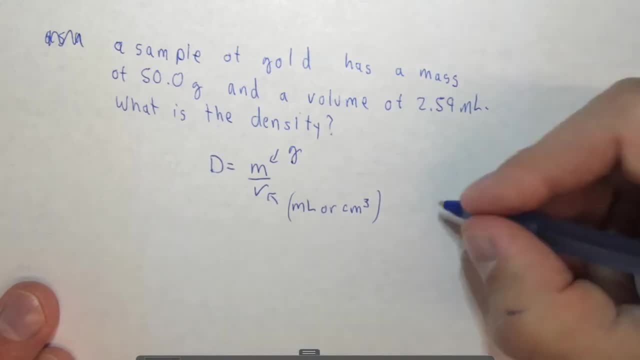 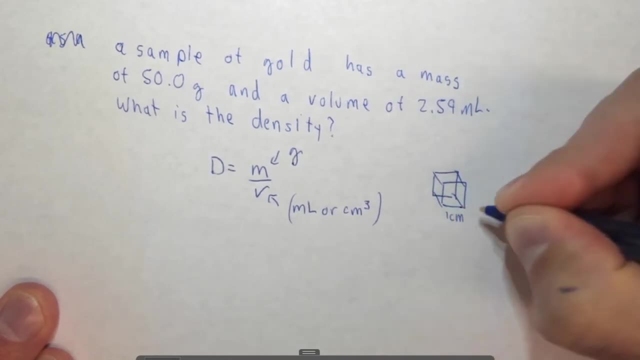 and a centimeter cubed or cc are the exact same thing, As I mentioned before. a centimeter cubed, that's one centimeter by one centimeter, by. it's hard to see here, but this back one, one centimeter. 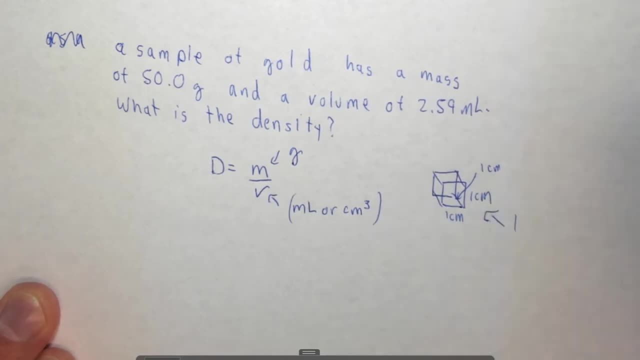 then this holds one milliliter of volume. So one centimeter cubed is a milliliter. So sometimes your units are in milliliters, sometimes they're in centimeters cubed. Some books will say this is for liquids and this is for solids, but I've seen both used. 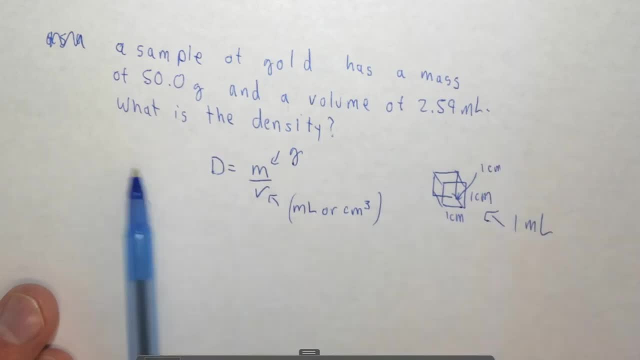 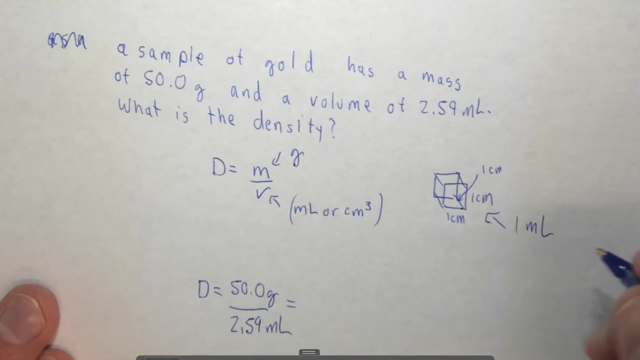 interchangeably. So back to the original problem. We're given a mass and we're given a volume. So density equals the mass- 50.0 grams, divided by the volume- 2.59 milliliters. So in this case we get 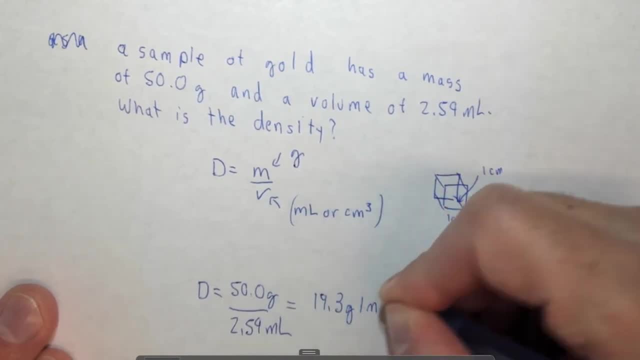 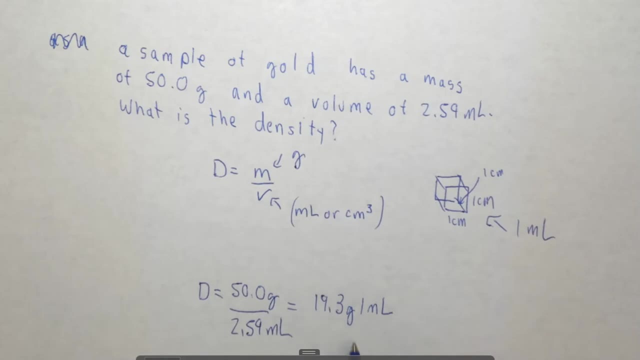 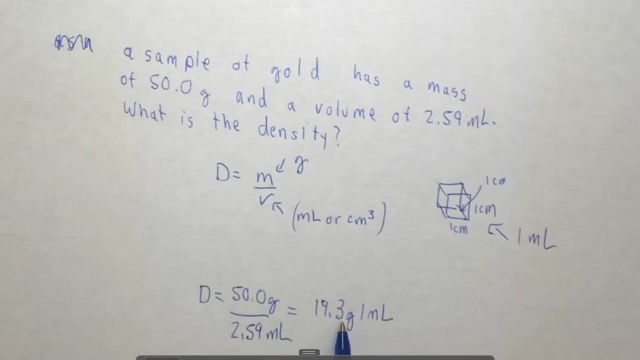 19.3 grams per milliliter. So gold has a density of 19.3 grams per milliliter, And this is constant. It doesn't matter at a certain temperature, it doesn't matter where the sample of gold comes from. 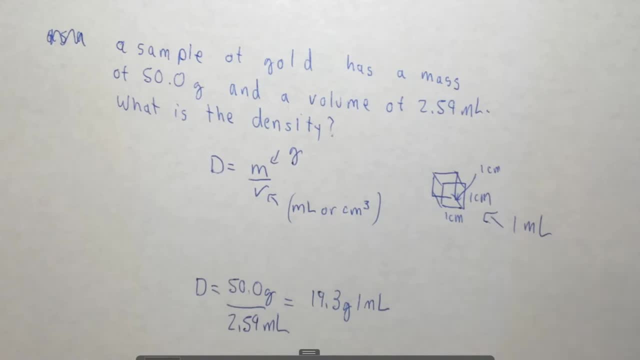 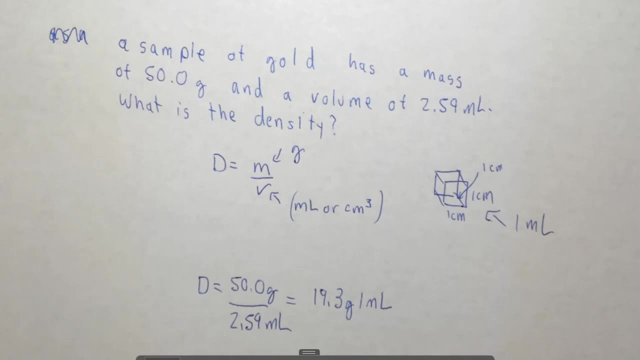 it doesn't matter if the sample of gold is from the United States or from China or wherever. it doesn't matter. Gold has a density of 19.3 grams per milliliter And this is one of the most dense substances on Earth. 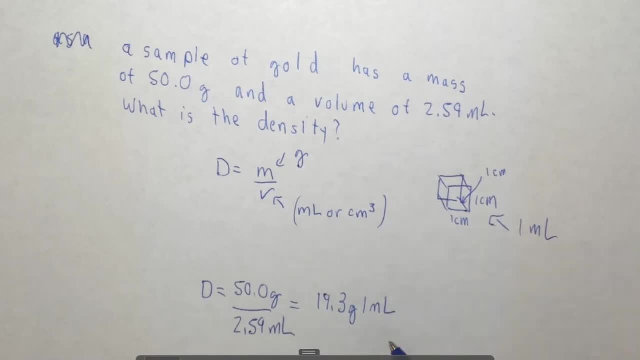 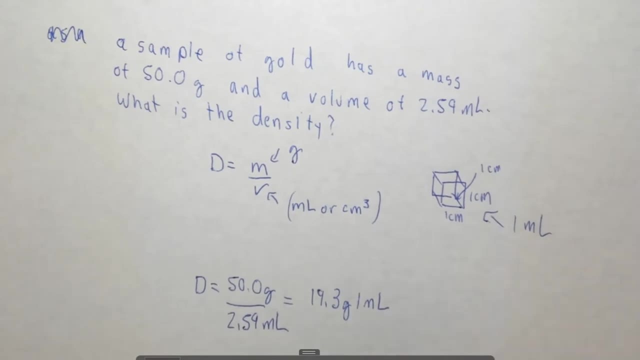 And, in fact, density was invented when people were trying to figure out whether crowns or other things that were supposed to be made out of gold actually were made out of gold, And one way to identify gold is through incredibly high density. If you use a, 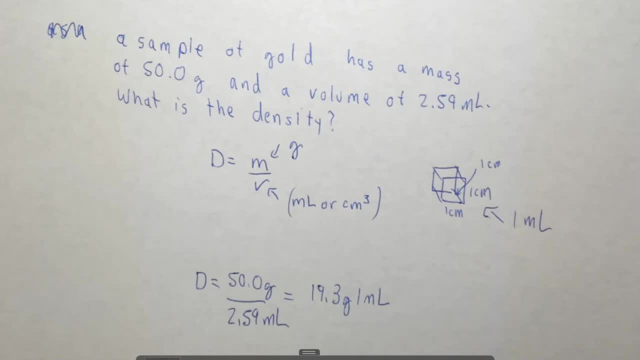 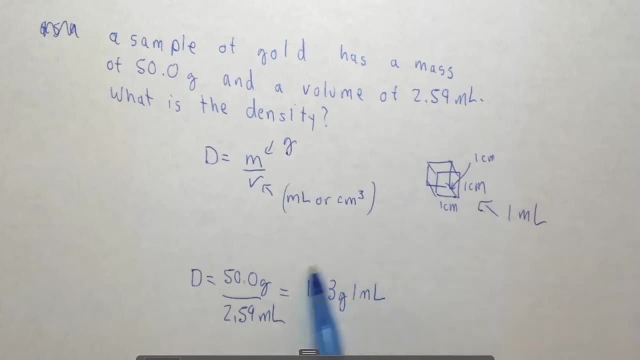 different metal, such as silver. it has a much lower density and that makes it distinguishable from gold. So if you measure the mass of the object and you measure the volume of the object if it's made out of gold, the ratio of the mass. 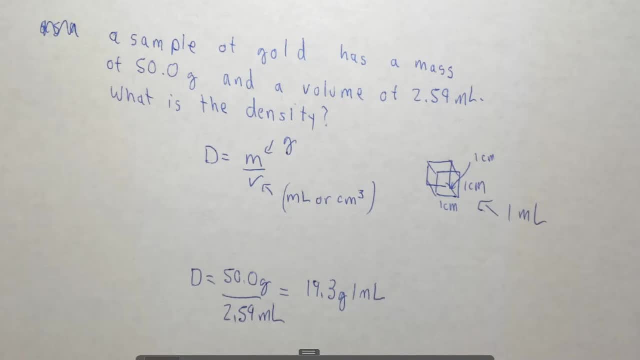 and the volume will be 19.3 grams per milliliter. Density is a good thing to calculate because it kind of ties together several of the concepts we're going to learn in this chapter. So in later videos in this chapter we will talk a little bit more about how we 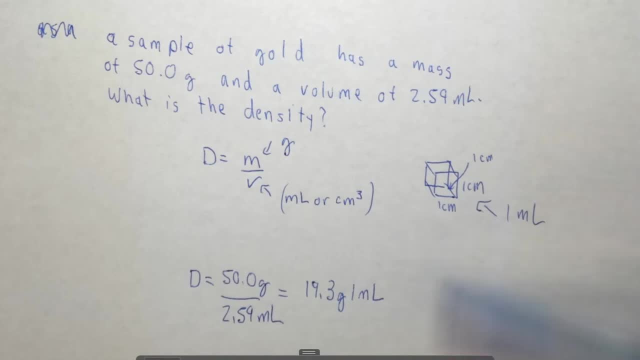 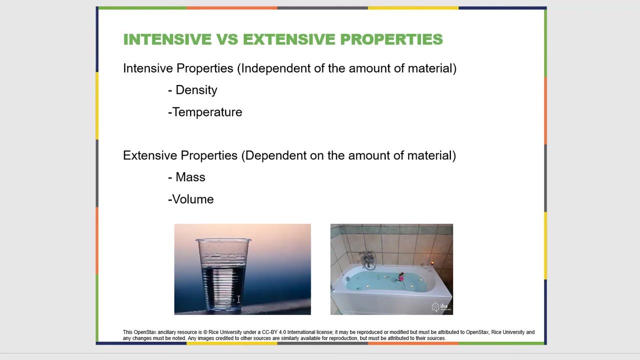 could actually calculate the density of the object and take into account things like significant figures and making accurate measurements and things like this. The last thing that I want to mention in this section is the difference between intensive and extensive properties. So intensive properties are properties that are: 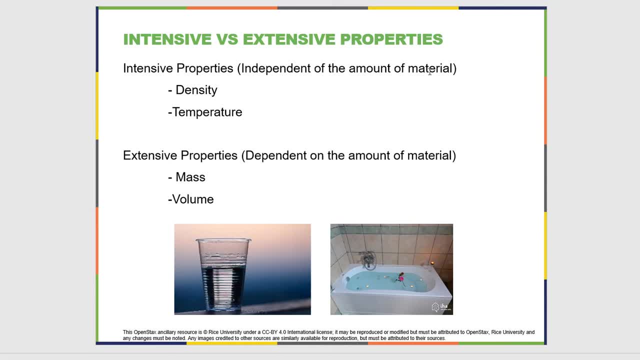 independent of the amount of the material. So it doesn't matter how much material we have- And we just mentioned densities in intensive properties. It doesn't matter where the gold comes from. Its mass to volume ratio is constant. If we look at water here: 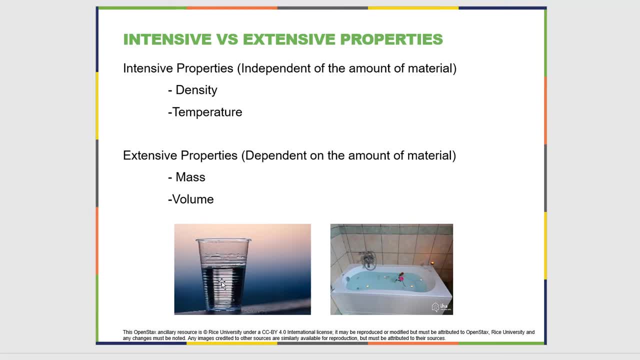 so say. this is a bathtub full of water and this is a cup of water that came from this bathtub. the density of this water in the cup is one gram per milliliter. The density of this water in the bathtub is still one gram per milliliter. 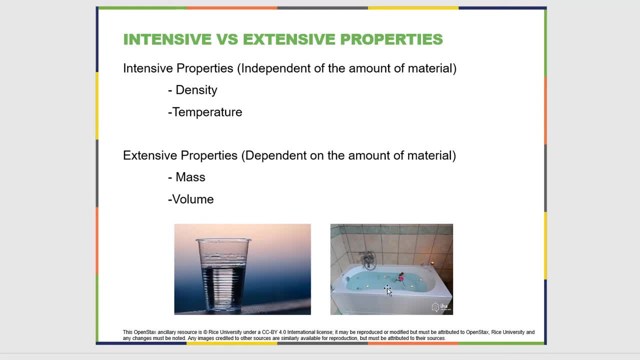 There's a lot more milliliters, but there's also a lot more grams. There's a lot less milliliters here, but there's also a lot less mass, So the densities are constant. Temperature is another intensive property that's independent of the amount. 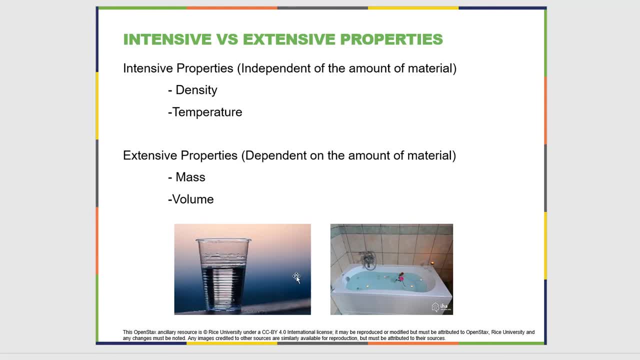 of the material. If this water is at 20 degrees Celsius and it came from this bathtub, which is also at 20 degrees Celsius, that would be a cold bath. That's room temperature. A bathtub would probably be closer to 38 or 39 degrees Celsius. 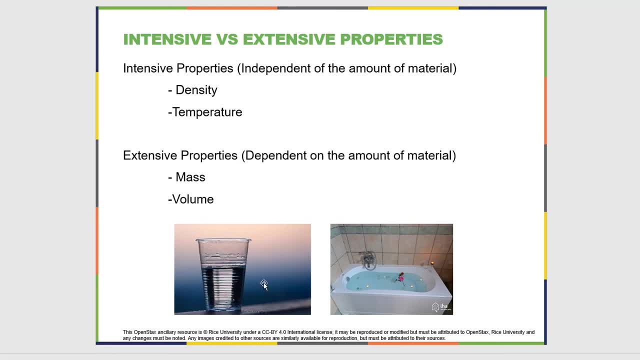 But in this case these things would have the same temperature. So it doesn't matter if the sample is in the bathtub or in the cup. They have the same temperature. So that's an intensive property. Extensive properties depend on the amount of the material. 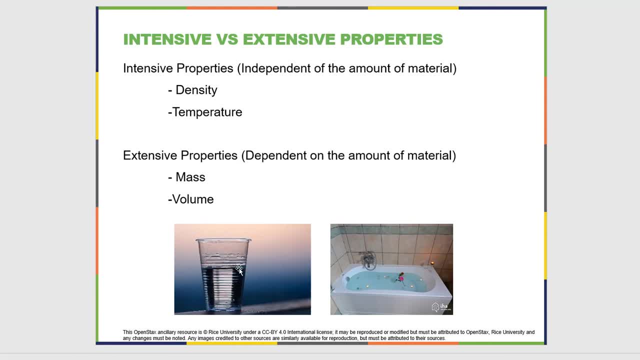 The mass of water in this cup is far less than the mass of the water in this bathtub. The volume of water in this cup is far less than the volume of the water in this bathtub. So these are extensive properties because they depend on how much you have. 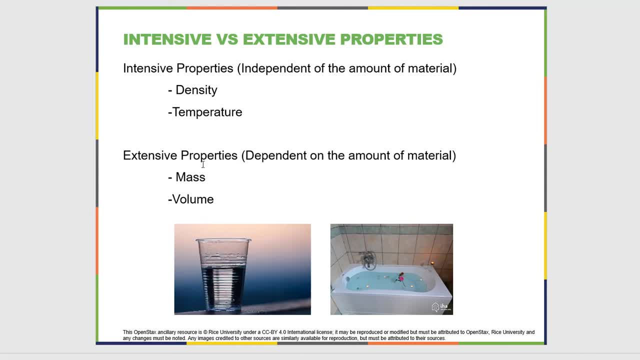 Less water means less mass and less volume. The final thing I want to mention as we conclude the video: If you notice, whenever we make a measurement we put a unit at the end, And in the lab as well as in the course.